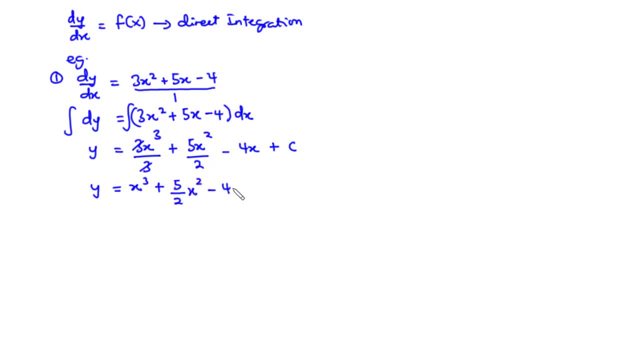 over 2 x squared minus 4x plus c. So this is what we have as equation for y. So y equals x cubed plus 5 over 2 x squared minus 4x plus c. Again, let's try this. Let's say you have the differential. 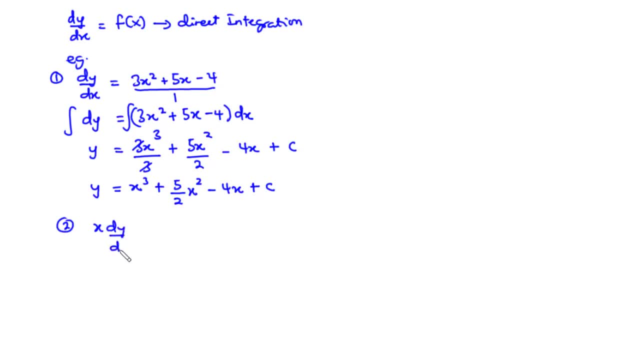 equation: x times dy dx equals 2 minus 4x cubed. Now also for this. the first thing you are going to do is to divide through by x. So you divide through each term by x, You are going to have dy dx to be equal to 2 over x minus. here x cancels one of the x's. 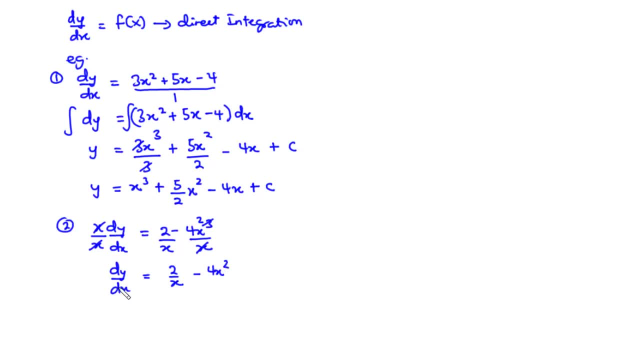 So you are left with 4x squared. Now you cross, multiply, you have dy equals 2 over x, minus 4x squared, or multiplying the x. Now you integrate both sides of the equation and then you have y was. Now you have this to be 2 over x. Now, because this is a constant, you can pull out. 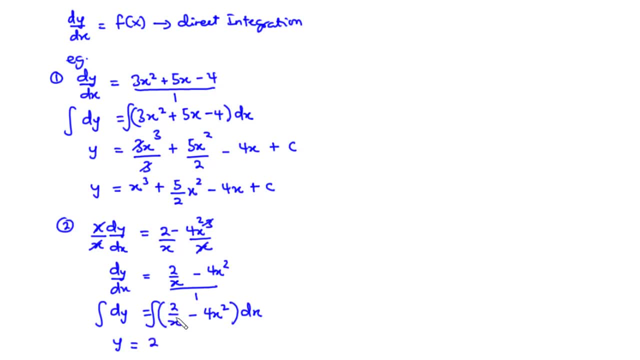 the constant, and then you are left with integrating 1 over x. Now, when you integrate 1 over x, you have ln of x, So that becomes 2 times ln of x minus. this becomes 4x cubed over 3. 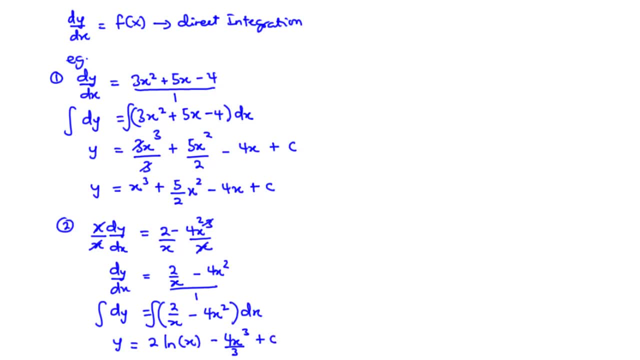 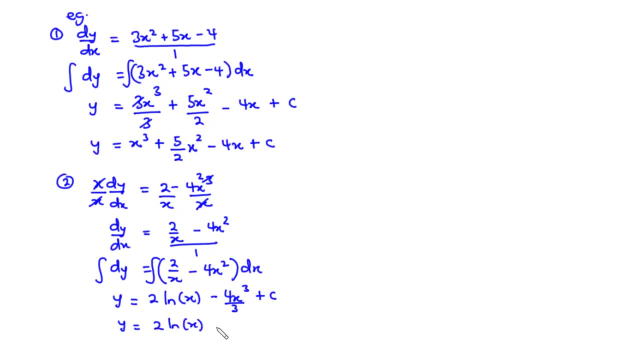 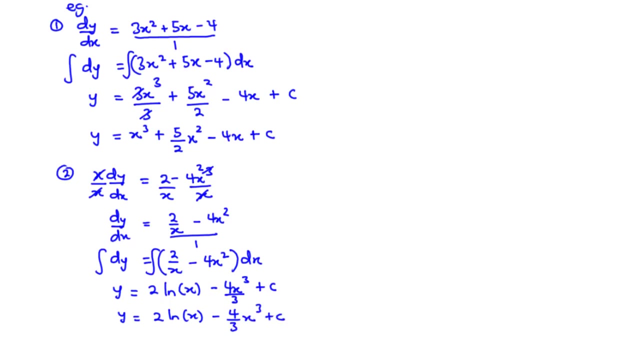 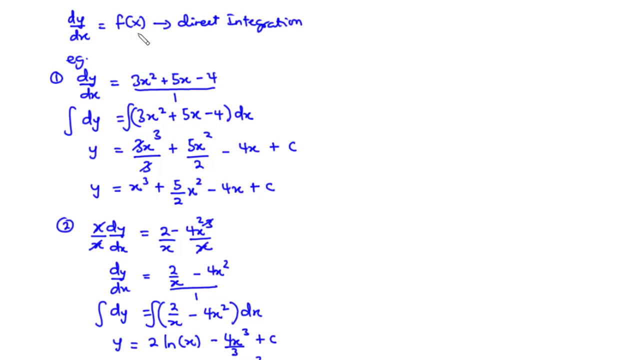 plus c. So finally you can have y equals 2 times ln of x minus 4 over 3 x cubed plus c. So basically this is how to solve differential equations given of the form dy: dx equals f of x. 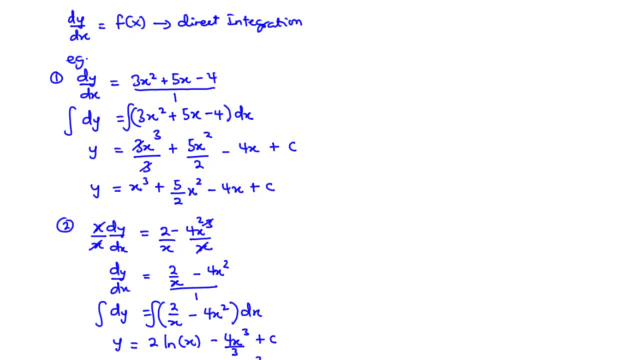 and that is by direct integration. Now let's move away from this. We focus on our main concern for today's lesson. So our main focus is to look at how to solve differential equations given of the form dy. dx equals f, of x, comma, y. Now here we have f to be. 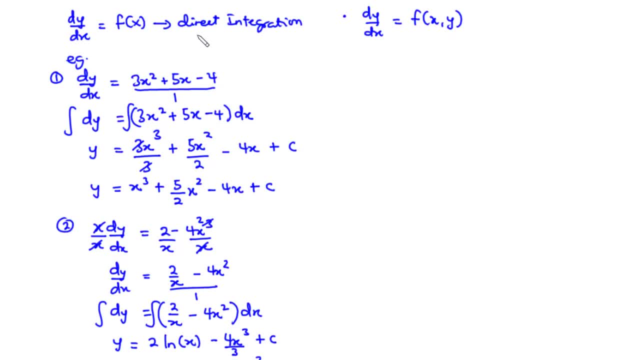 a function of x and y. So in this case, direct integration is not going to work, and so we need to use a different approach. So, given the differential equation of the form dy, dx, we are going to use f to be a function of x. equals f of x comma y. Now if this differential 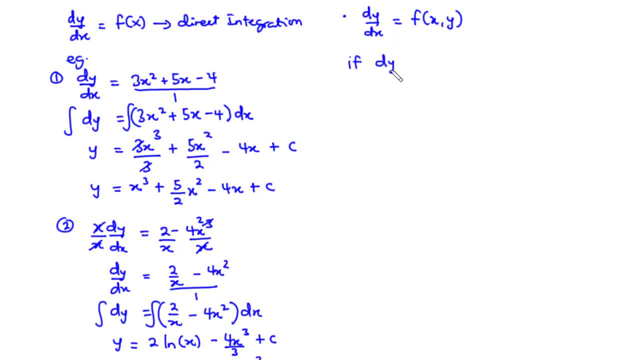 equation. if the differential equation can be expressed as the product of two functions, that is, the product of h of y and g of x, where h is a function of y and g is a function of x, Then we say that this type of differential equation is a variable, separable type. 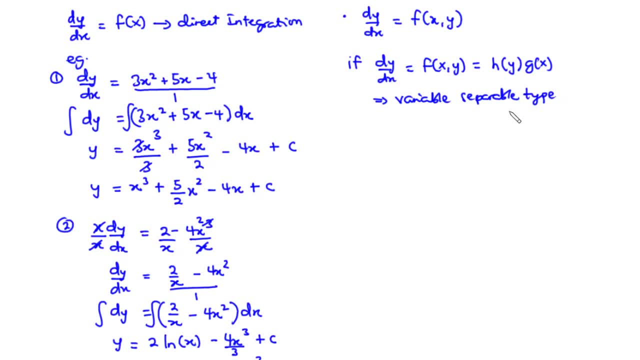 Then the differential equation is a variable separable type And, more importantly, if h of y is not equal to 0, then what we can do is to separate the variables by grouping all x's on one side and then all y's on the other side. 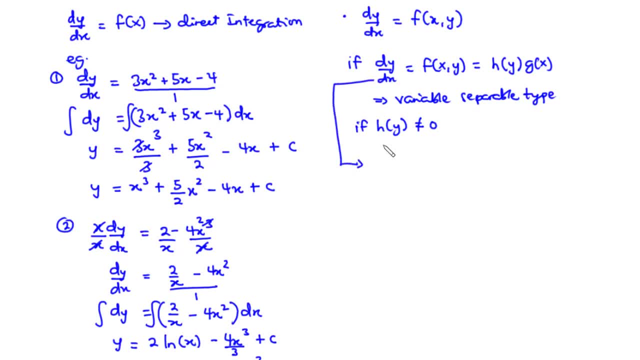 So from this we are going to have dy, dx equals. now we eliminate this and then we have the product of h of y And gene of x. So we cross, multiply, We have dy equals h of y times gene of x or dx. 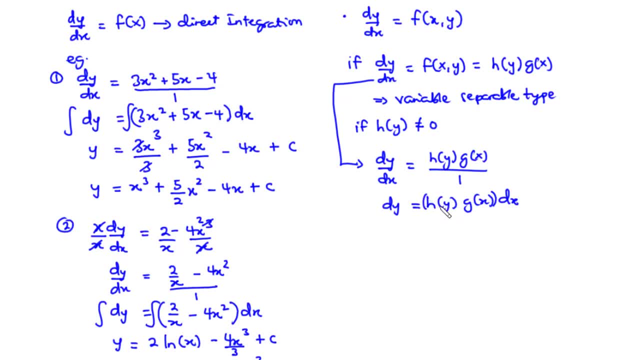 So all times dx. And because here we have a function of y, we need to divide through by h of y. So we divide through by h of y And then we are going to have 1 over h of y. dy equals gene of x, dx. 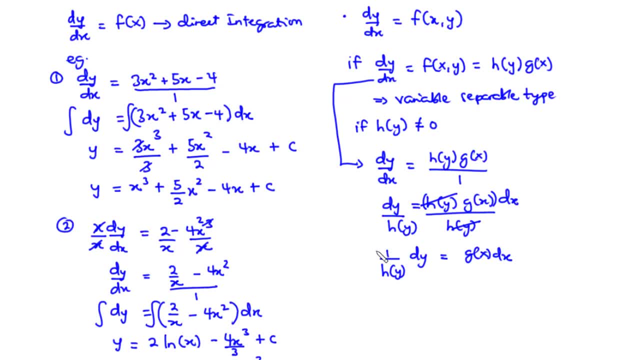 Now, at this point we are going to integrate both sides. So we integrate both sides, and then we are going to have capital H of y equals capital gene of x plus c, Where capital H of y and then capital gene of x are integrals of 1 over small h of y and then small gene of x. 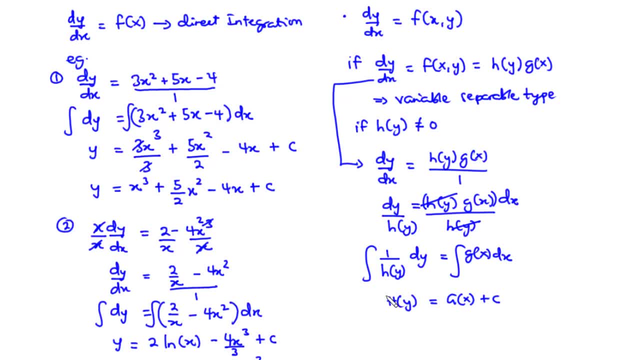 And then c is said to be the arbitrary constant, And this equation is called the general solution to the given differential equation. So this happens to be the general solution to the given differential equation. Now, one important thing we need to take notice of is that every type of differential equation has its own way or method in solving. 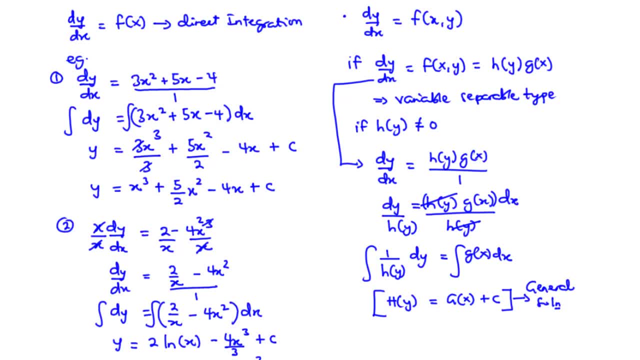 So it is our responsibility to know the type of differential equation given before we know which method to use. And, most importantly, this information will not be given in our exam or on our exam sheet. And so it is our responsibility, as I said earlier, to know which type of differential equation you are dealing with and which approach. 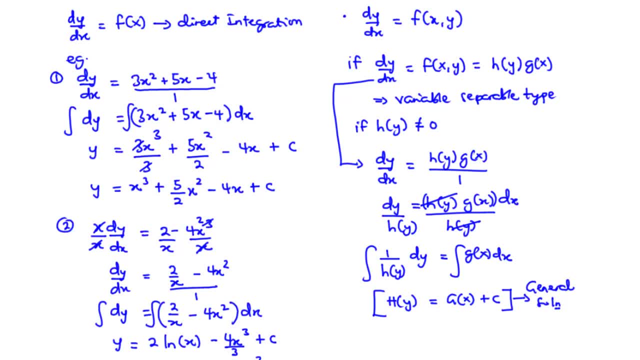 Or which method you are going to use or apply Now. at the moment we've been able to know that or understand that for a given differential equation of the form dy, dx equals f of x, you can solve by doing direct integration. However, when you are giving a differential equation of the form dy, dx equals f of x, comma y, where f is a function of x and y, 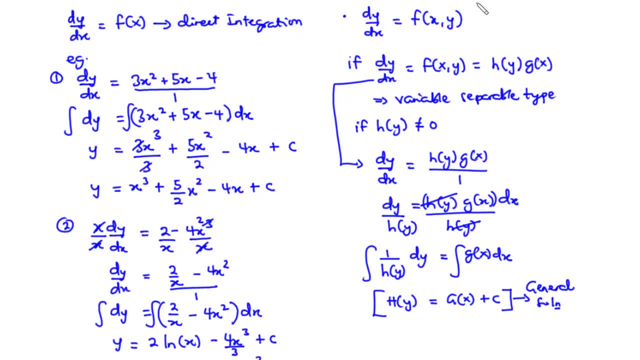 you need to solve that by separating the variables. So if you have something like this, then what we are going to do is to solve by separating the variables. Hence this type of differential equation is called separable differential equations, And because we are dealing with first order, first degree differential equations, 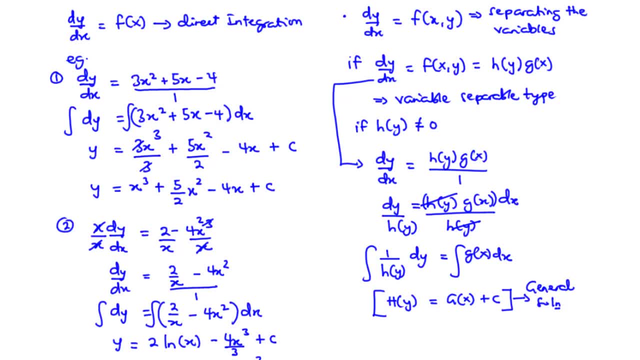 then this becomes a first order, first degree differential equation. Then this becomes a first order: first degree differential equation, Separable differential equation. Now let's move ahead as we solve a couple of examples. So let's take our first example. 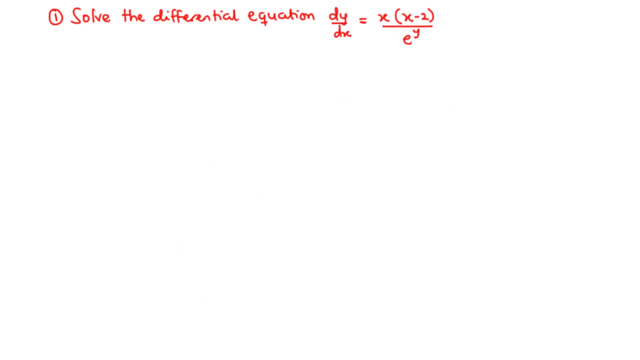 In this example we are going to solve the differential equation. dy dx equals x times x minus 2, or divided by e to the power y. So let's do this together. So we have dy dx equals x times x minus 2.. 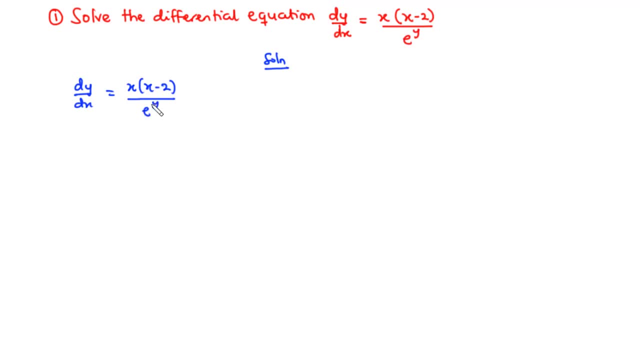 2, all divided by e to the power y. now, looking at this differential equation, you realize that here we have a function of y, and so direct integration is not going to work. hence we need to solve this differential equation by separating the variables. so the first thing, 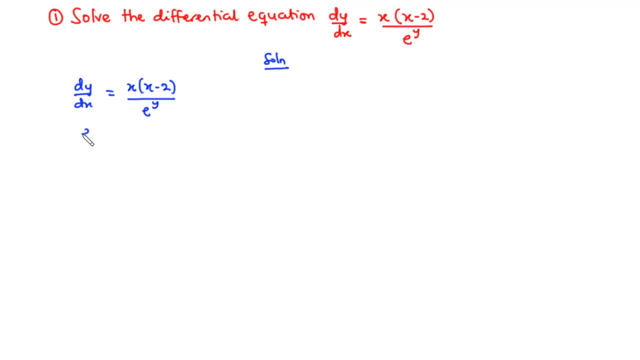 we are going to do is to cross multiply, and so we are going to have e to the power, y times the y, and that's equal to. simultaneously, let's expand, so we have x times x, which is x square minus 2x, and then we have all this multiplying the x. now we've been able to separate. 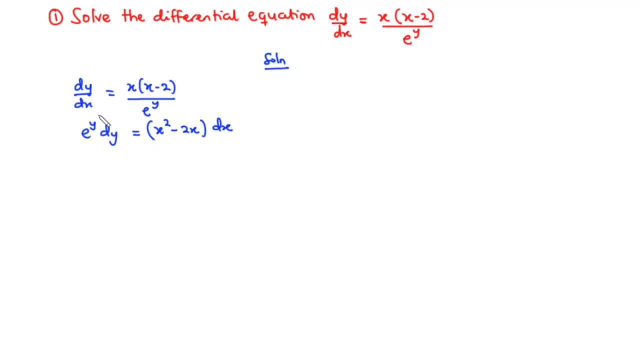 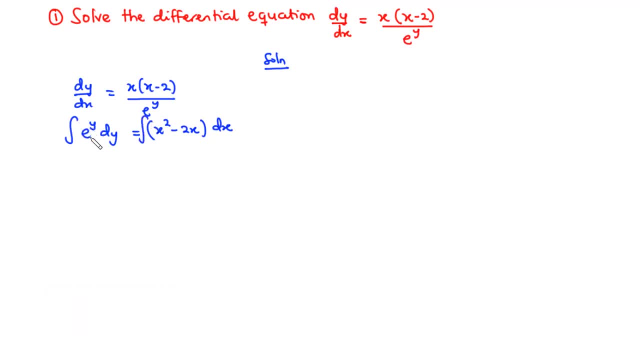 and then we have now, when you integrate e to the power y, you still have e to the power y and that is equal to: on the right hand side we have x cube divided by 3 minus 2x square divided by 2 plus c. so this becomes e to the power y is equal to x cube over 3 minus. 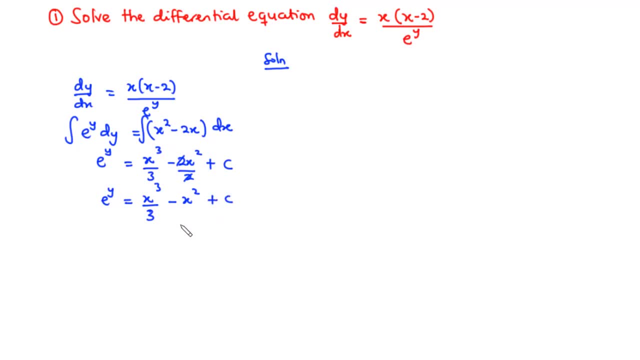 x square plus c. now, since you are supposed to solve for y, then it means we are going to introduce the natural log, so we can represent this equation as ln of e to the power. y equals ln of x cube divided by 3 minus x square plus c. now at this point you realize that 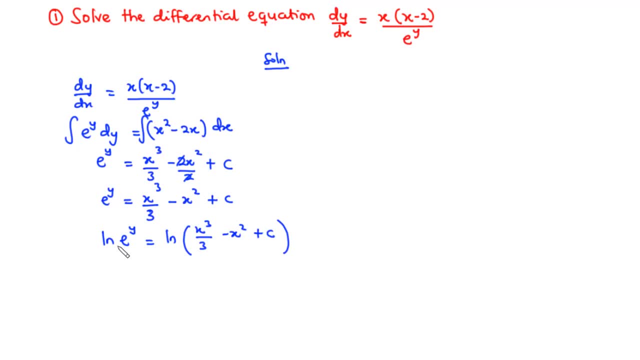 our log has a base of e. so we say that ln of e to the base, or, better still, ln of e to the power, y to the base, e, and then we are going to transport this y or this exponent to be in front of the log. so basically we have y times ln of e to the base e. now log. 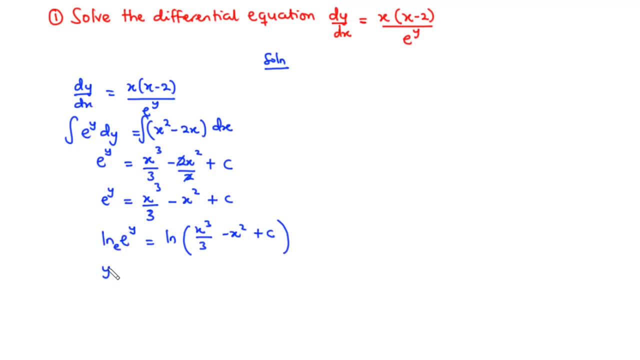 of the same base is equal to 1. therefore, y times 1 is still y. so y is equal to ln of x cubed over 3 minus x squared plus c. Hence we've been able to solve for y. So, basically, this is how to solve this question. So let's move on to the second example. 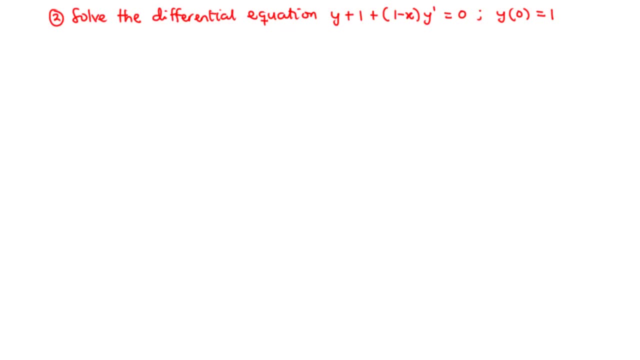 So, for example, 2, now this time let's try a more complicated one. So we are going to solve the differential equation y plus 1 plus into brackets 1 minus x. all multiplying y prime equals 0, where y of 0 is equal to 1.. So here we are, given the differential equation, and then it. 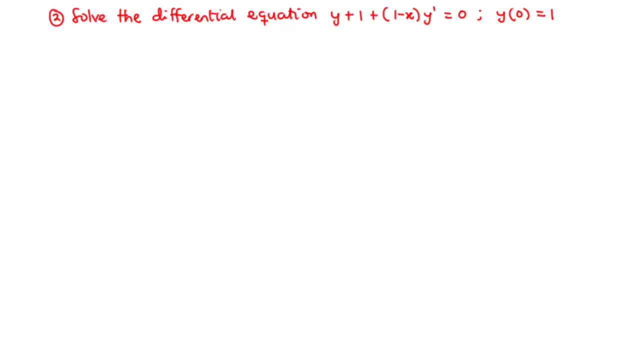 comes along with a condition, And so, basically, what you are going to do is to solve for the particular solution for this differential equation. So let's do that together So we can repeat. Let's represent this differential equation as y plus 1 plus 1 minus x, all multiplying dy, dx. 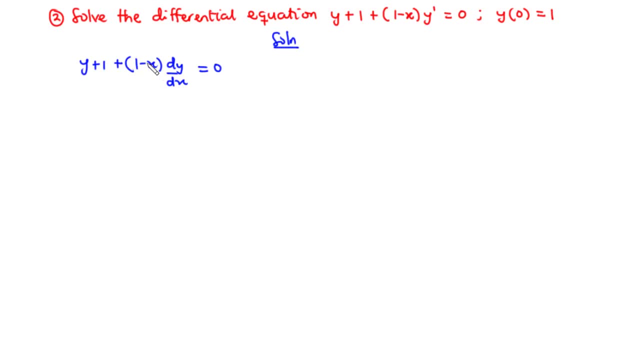 equals 0.. Now let's transpose this term to the right-hand side. So we are going to have y plus 1 equals negative, 1 minus x, dy, dx. Now we can multiply negative. Let's imagine that we have y plus 1 plus 1 minus x, So we are going to have y plus 1 plus 1 minus x. 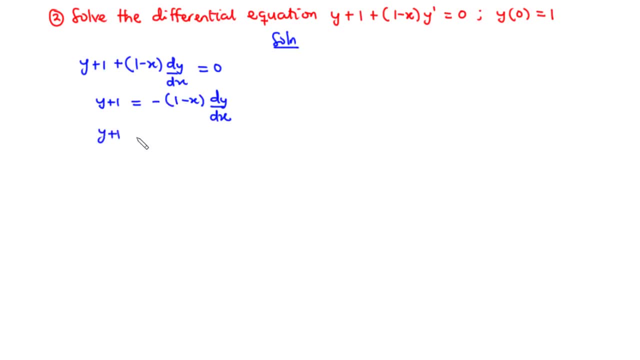 negative 1 across, so it becomes y plus 1 equals now negative 1 times 1 is negative 1, so we have negative 1 and then negative 1 times negative. x is plus x, so we can represent this as x minus 1. so we have into bracket x minus 1, dy dx. at this point we have x here, we have the x here. 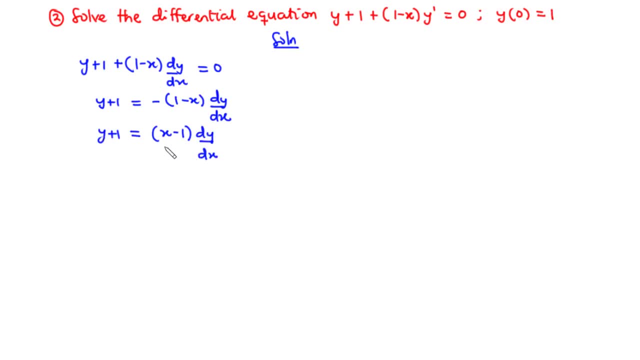 we have y here, we have dy here, so we can choose to divide through by dy. so when we do that, this cancels out this, and then we are left with y plus 1 over dy equals x minus 1 divided by the x. so we can flip this equation on both sides. so 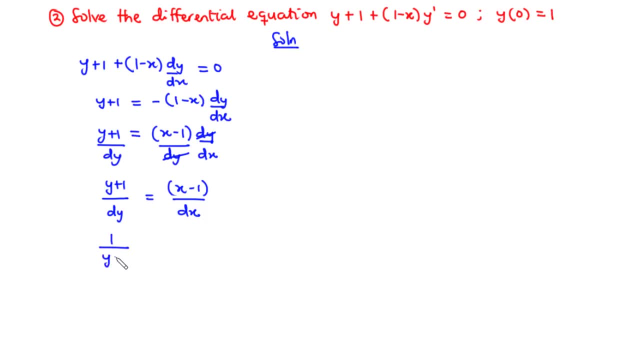 that we have 1 over y plus 1 all times dy equals 1 over x minus 1 all times the x. so at this point we can find the integral of both sides, and so when you integrate 1 over y plus 1, then you have ln of y plus 1 and that is equal to the same applies. here we have: 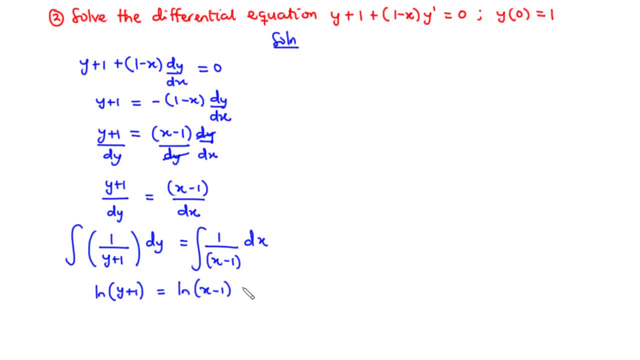 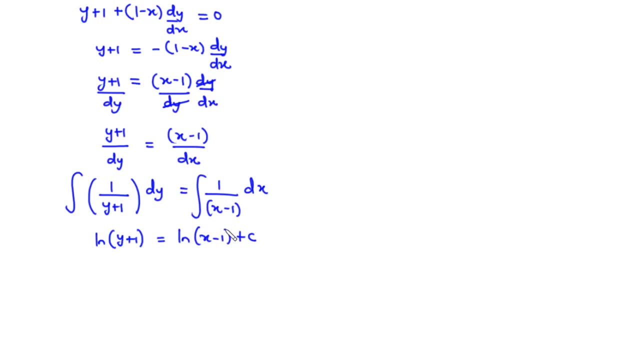 ln of x minus 1 plus c. now, at this point, what you are going to do is you are going to transpose ln of x minus 1 to the left hand side, so that becomes ln of y plus 1 minus ln of x minus 1 equals c. 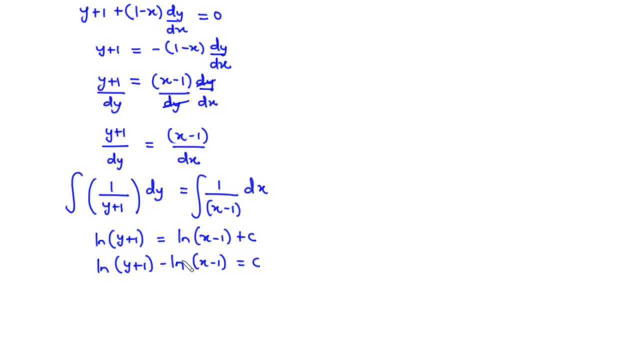 now, because we are subtracting two logs. then, using the properties, it means that we are going to divide. so we have ln of y plus 1 divided by ln of 1 plus, rather than wi- 안돼 for x minus 1. so the moment you are subtracted, you are going to. 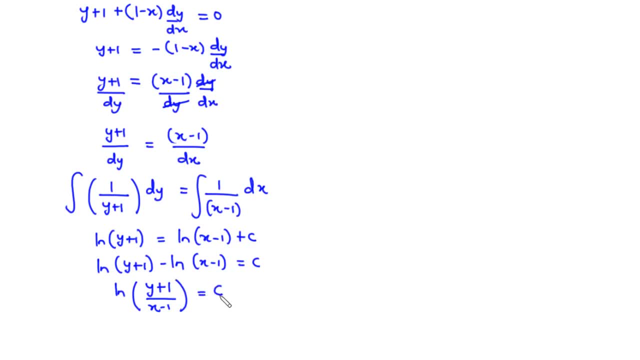 divide. if you are added, then it means you are going to multiply. so that is equal to c. now, at this point we know that the natural log has a base of e. so we have ln of this to the base e and using properties, we can have a new equation by removing the log or ln, that is, by transporting c 2x minus 1 to crazy himsины, the power solution we obtaining the value of, and little f is divided into zero. no, both factor is to the base of e, that's our. so we have ln of this to the face e and using properties, we can have a new equation by removing the log, or ln, that is, and using properties. we can keep the equation by removing the log or ln. 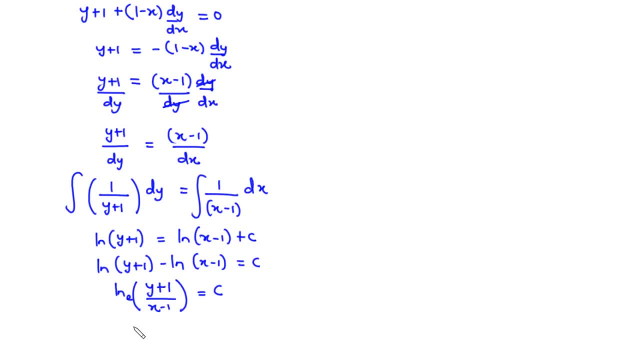 on e, and that will be equal to this term. so that becomes: e to the power c equals y plus 1 over x minus 1. so by this we've been able to eliminate the natural log, and so we have e to the power c equals y plus 1 over x minus 1. now at this point we can cross multiply. so when we cross multiply, 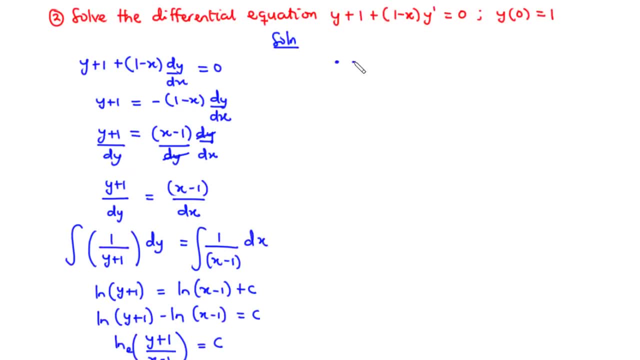 then we are going to have e to the power c times x minus 1 equals y plus 1. and then, because we want to solve for y, we transpose 1 to the left hand side. we have e to the power c times x minus 1 minus 1 and that is equal to y. now you need to understand that e is a constant. 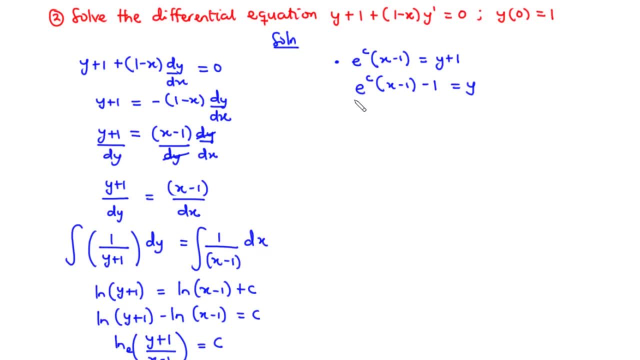 and then c is also a constant. so to simplify this equation, we can say that: let e to the power c equals c1. now, because e is a constant, and then it is raised to the power a constant. it means that if you want to simplify this, your answer is going to be a constant. so at the end, 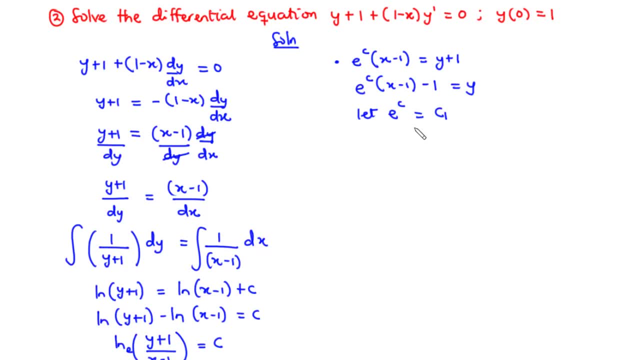 you are going to arrive at having a constant, so it is better to make e to the power, c be another constant, let's say c1. so at this point you are going to have y to be equal to. you have c1 times x minus 1 minus 1. so this is called, this is called the general solution. the general solution. 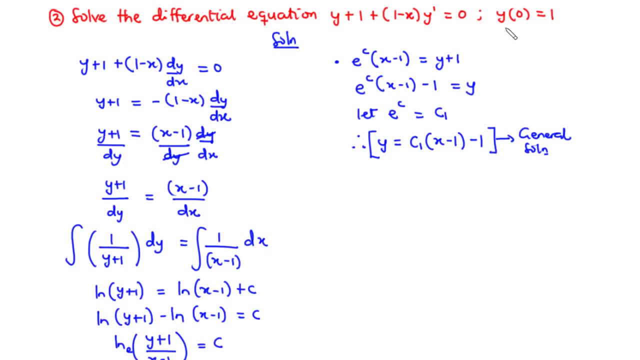 to the differential equation. now we are given an initial constant condition, that is, y of 0 equals 1. so at this point you know that x is equal to 0 and then y is equal to 1. so let's plug in these values in place of x and y in this general solution. 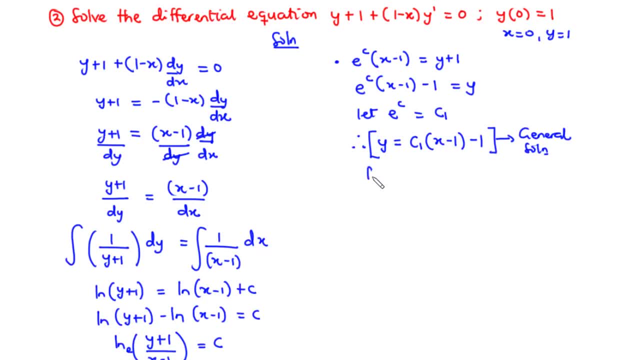 so for y we have 1, so we say that's 4 for x equals 0, and then y equals 1, we are going to have 1 equals c1, into brackets 0 minus 1 minus 1. so what we are going to do is to: 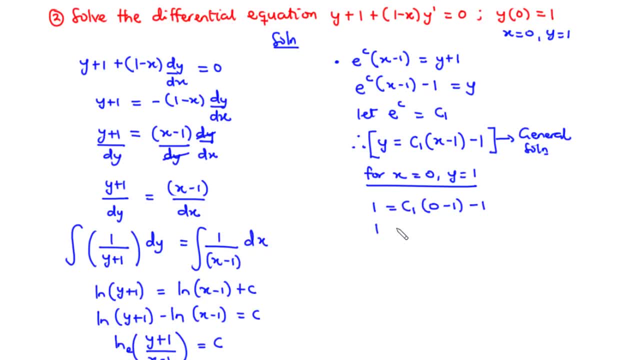 find the value of c1 so that becomes: 1 equals 0 minus 1 is negative 1, so negative c1 minus 1. we transpose this to the left hand side. we are going to have: 1 plus 1 equals negative c1. 1 plus 1 is 2 equals negative c1. we divide through by negative 1.